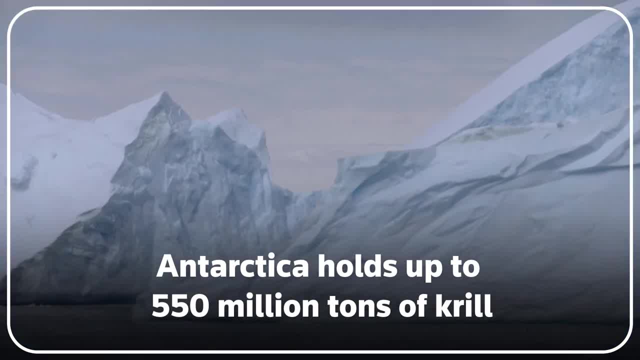 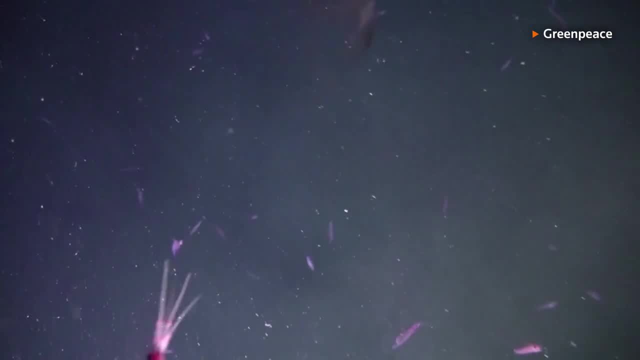 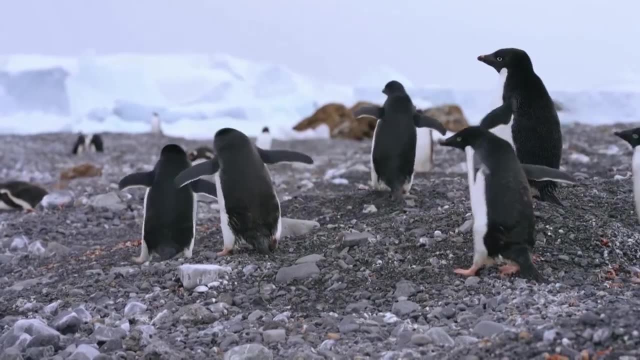 The icy waters of Antarctica are estimated to hold up to 550 million tons of krill. These tiny shrimp-like creatures are the linchpin in the Antarctic food web, sustaining a huge number of species from penguins to humpback whales. 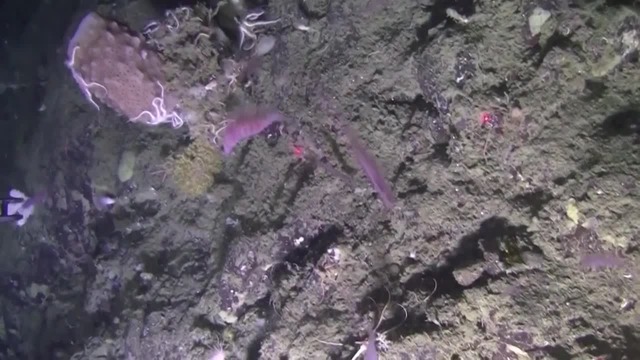 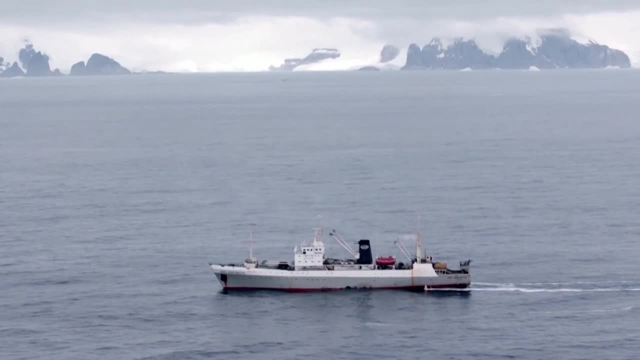 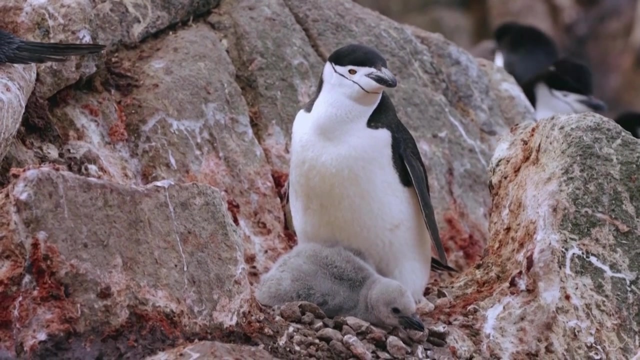 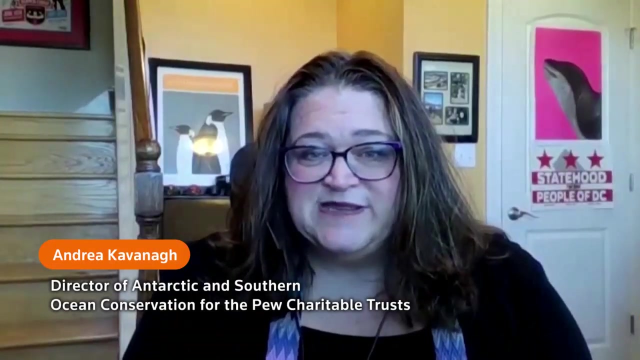 They are also increasingly the target for human consumption. A growing krill industry has been scooping up the crustaceans for use in fish oil supplements and fish feed. Scientists and conservationists fear that could further imperil Antarctic wildlife. Antarctic krill are the keystone species in the Southern Ocean. 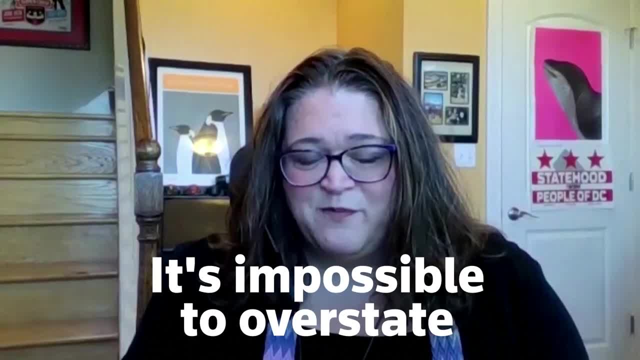 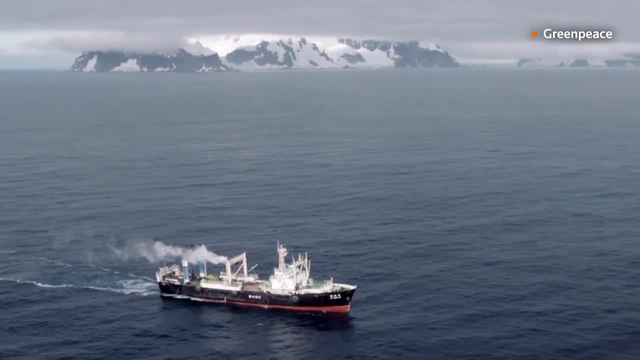 Krill connect all the other species down there. It's impossible to overstate the importance of krill. This perceived overpowering phenomenon has led global fishing fleets to target Antarctic krill Vessels from China, Norway, South Korea, Ukraine and Chile. 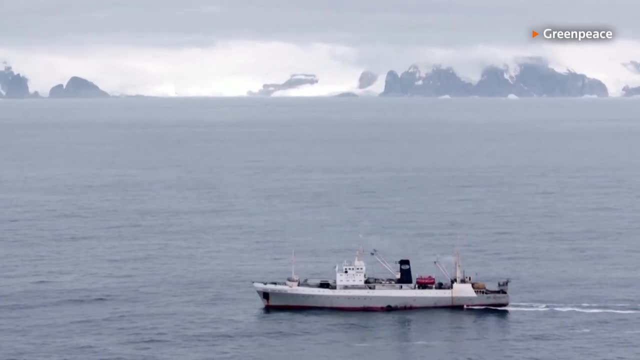 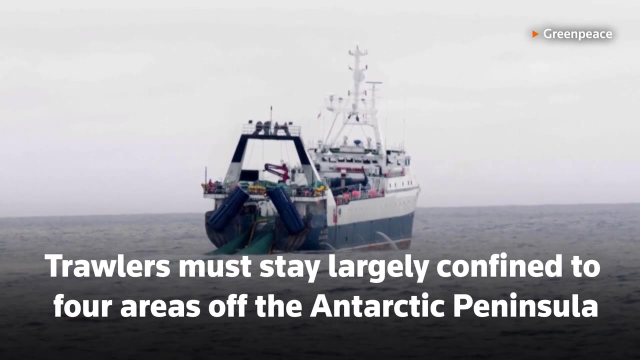 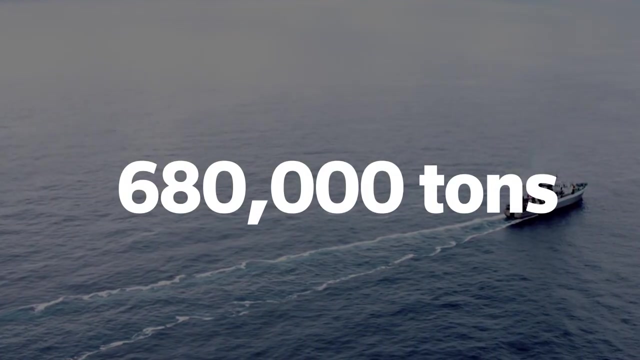 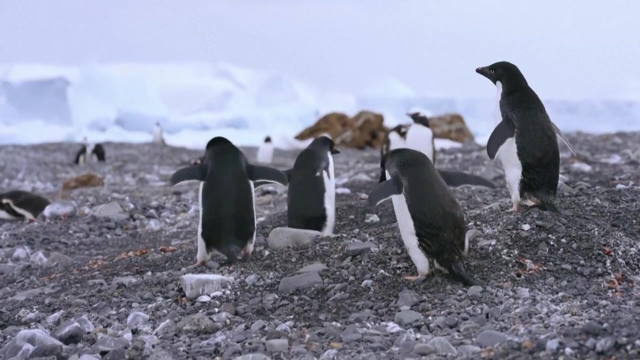 trawl the region's choppy waters from December to July. Under established rules within the Antarctic Treaty System, trawlers must stay largely confined to four areas of the Antarctic Peninsula And the seasonal catch is capped at 680,000 tons. But polar scientists say the current limits may not go far enough. 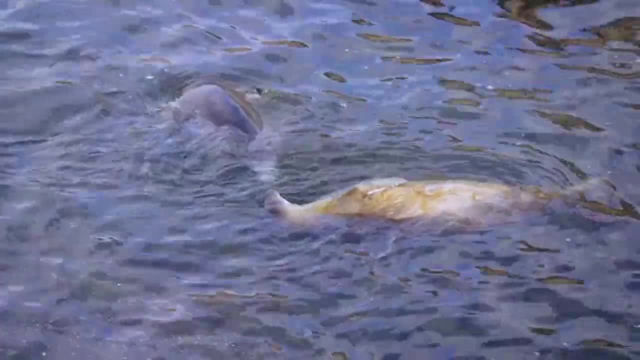 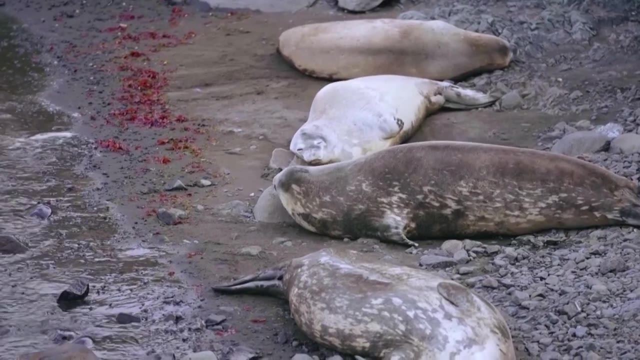 to safeguard the food supply for wildlife. Some also say there are indications that the fleet's activity is harming wildlife. For the first time ever, it was reported that there were bycatch in the krill industry of whales- Three juvenile humpback whales. 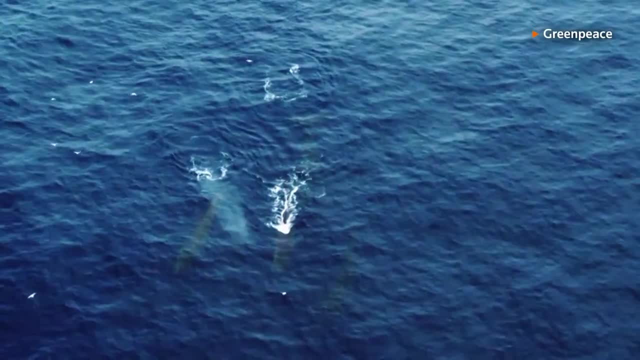 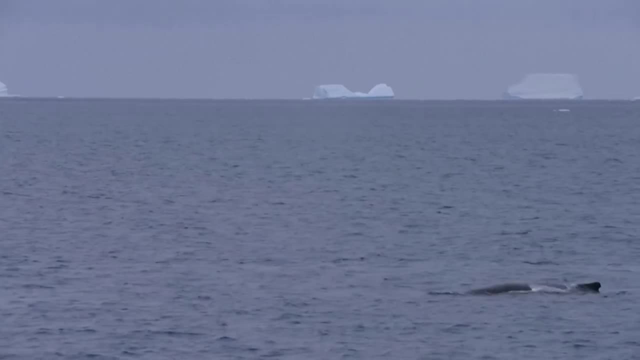 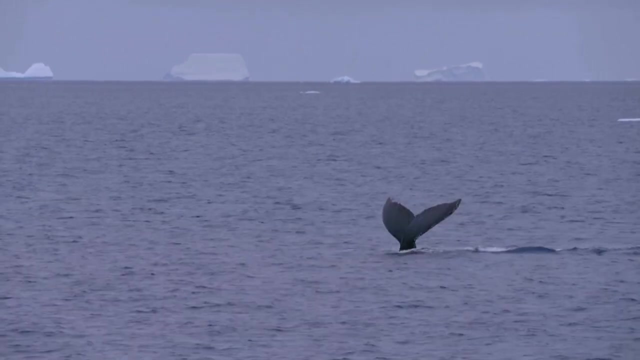 And it's actually unknown how they came about to be caught by these continuous suction trawlers. They were definitely in poor body condition, They were starving, So they suspect perhaps that the krill, that the humpbacks, were actually following the krill trawlers. 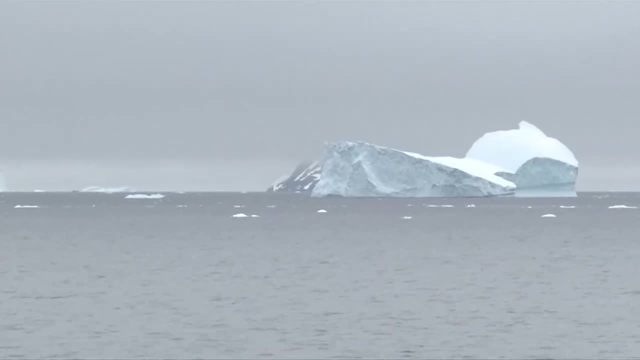 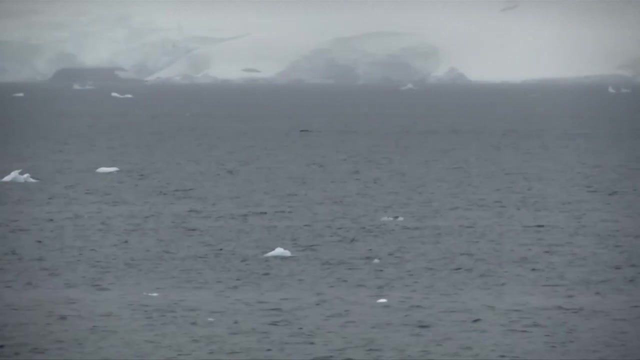 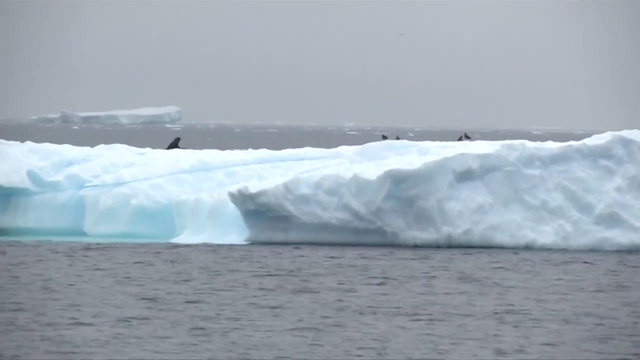 to try to get krill and somehow got caught up in their systems and nets. But it seems really troubling that there were actually three of them that were caught this year, when that's never happened before. The fishing company Norway's Akir Biomarin.